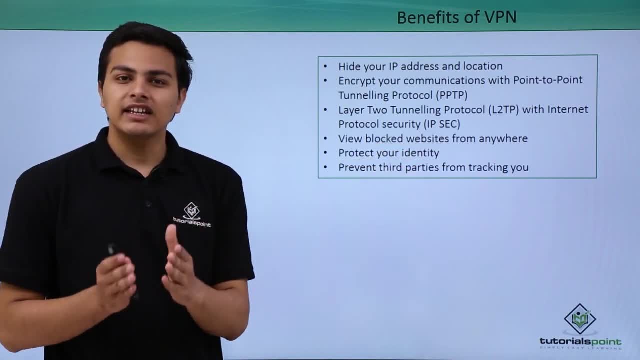 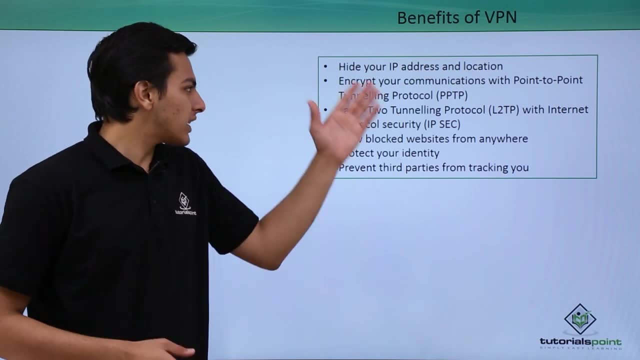 Then the third protocol which VPN uses is called IPsec, Say that internet protocol security. By using this protocol, VPN tries to secure our IP addresses. So these are the few techniques which VPN use in order to secure our communication and encrypt our communication. So then, another benefits of VPN are same like proxies. 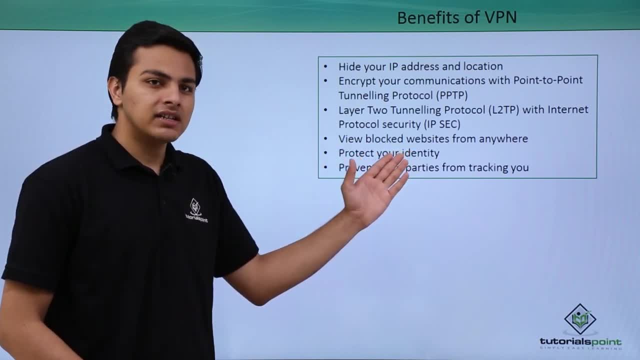 So these are the two most important things: which VPN type in order to secure and encrypt our communication? The three main benefits of VPN are same: like Proxie, like we can view the blocked website, we can change our IP address, we can protect our identity and the main benefit is that we can prevent third parties from 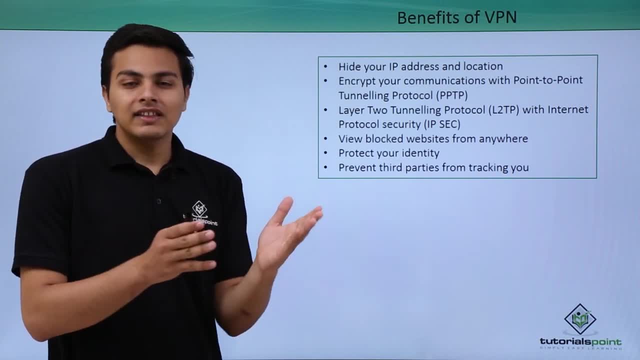 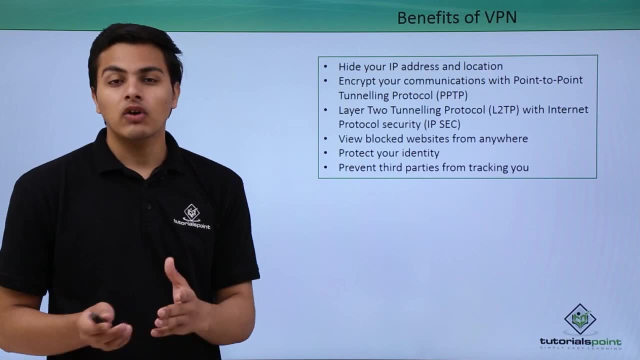 tracking us. so if our request is encrypted, then nobody can track us. nobody can figure out there what's present inside that request. now let's see how we can use CyberGhost VPN in order to see that how VPN works. now let's use CyberGhost VPN in order to see that how VPN works. well, first of all, we 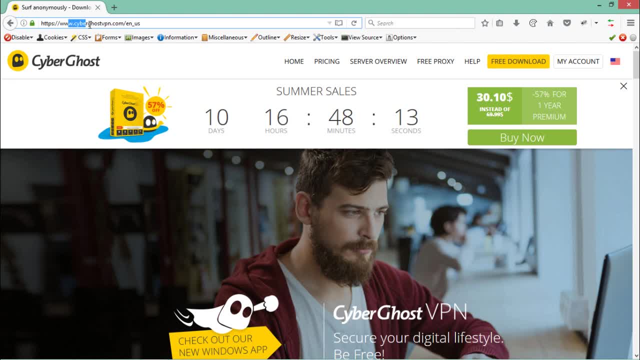 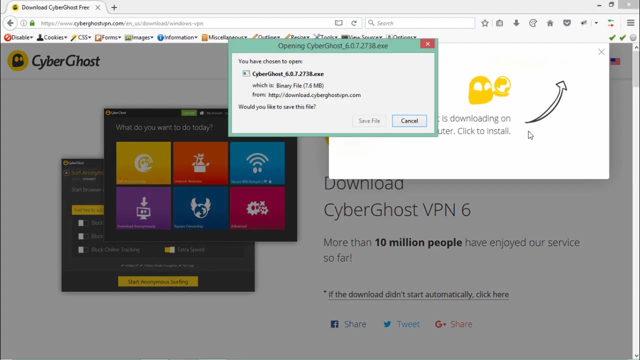 have to download the CyberGhost VPN, and you can download that VPN from here from this URL, CyberGhostVPNcom, and here you will see one link of free download. so let me click over here and let me save the executable file. so I personally recommend you to please use CyberGhost VPN in order to serve anything online. 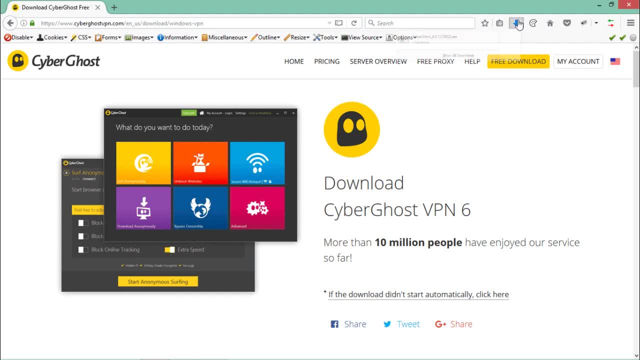 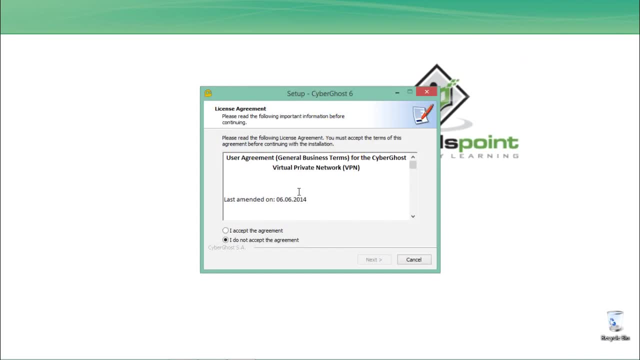 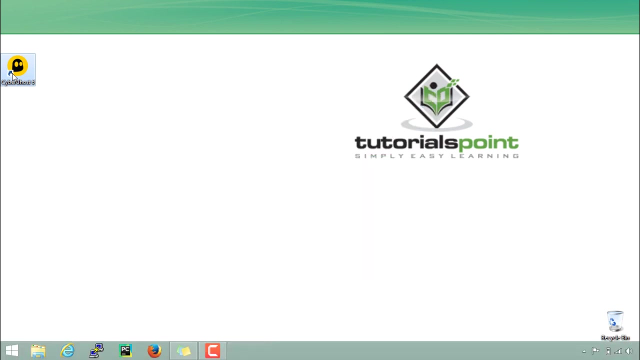 because this is the best VPN I have ever used, and let me install this so you can also buy the premium pack of this VPN. and once this VPN is installed, it will start running. and here you can see that on my desktop, icon of CyberGhost is created. 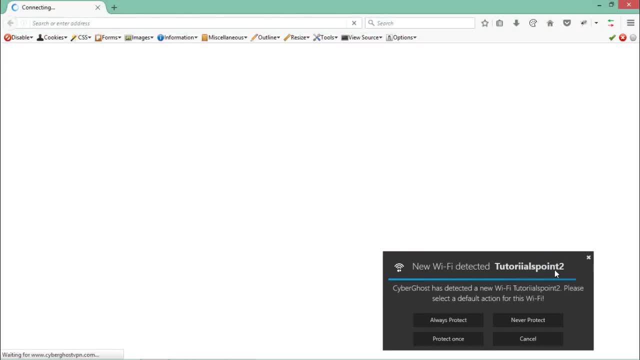 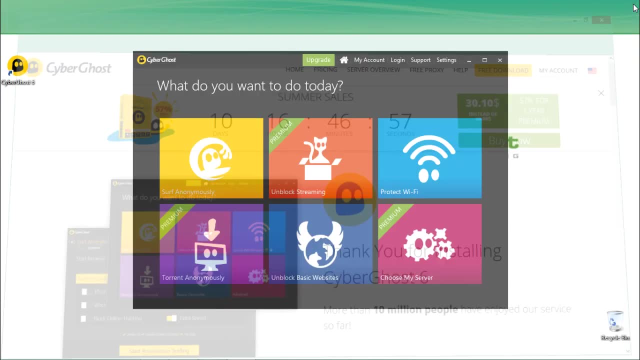 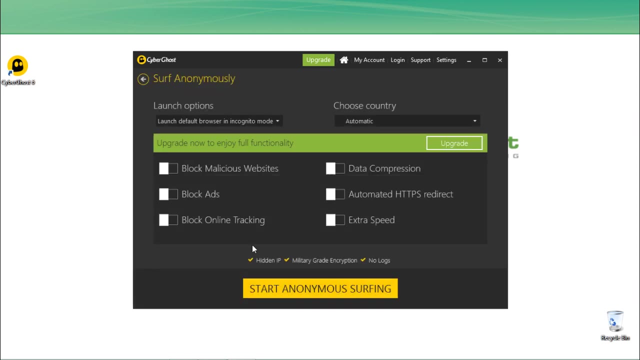 and here you can see the first of all. it will tell us with which Wi-Fi connection we are connected. and here is the advertisement. let me also close this thing. so here you can see the main menu of CyberGhost. there are a lot of options, so let's click over here, surf anonymous. click on start anonymous surfing and here we have to wait for few seconds. so this is a main limitation in the free version of CyberGhost: that we have to wait for some time in order to access this VPN. and here you can see that they are saying: all free users slots are booked. 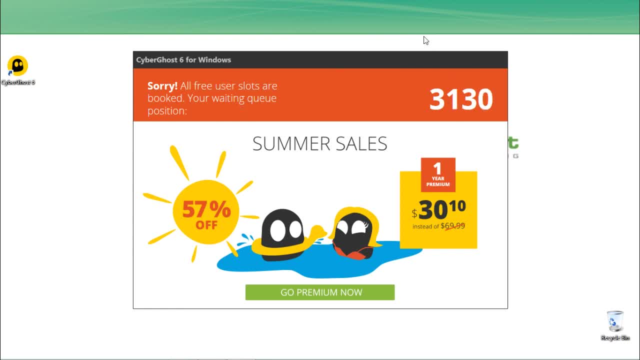 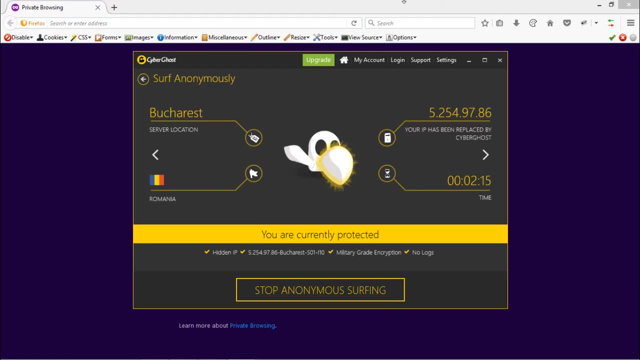 and your waiting queue position, and we have to wait for these few seconds and I'll resume the video once this seconds are over. now, here you can see that our CyberGhost VPN is up and running, here you can see the uptime. and now the CyberGhost VPN has replaced our original IP address and here you can see that the